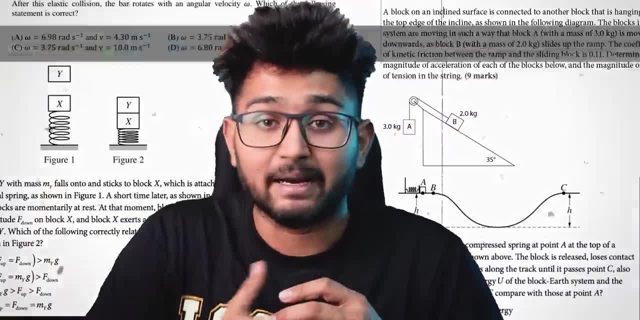 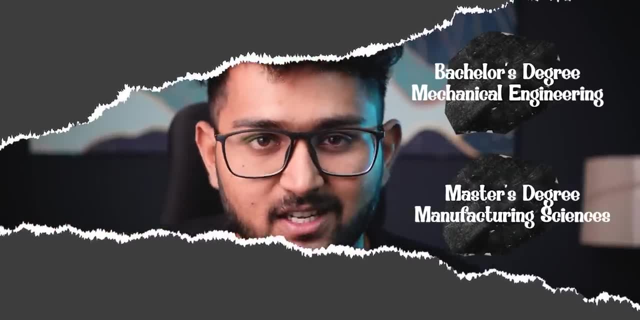 And back then my aim was to frame 5 questions which even my teachers won't be able to solve. So right from then to graduating from IIT Kharagpur with a bachelor's degree in mechanical engineering and a master's degree in manufacturing sciences, I read books after books and solved questions after questions. 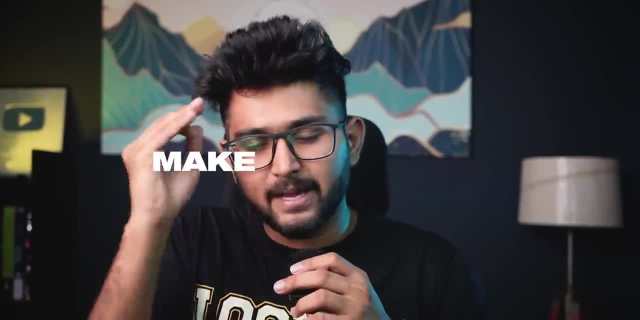 And I just love physics. So let me tell you, in the next 8 minutes of your life, I'll make you fall in love with physics And, most importantly, we'll give you a step-by-step guide to master it. Let's start. 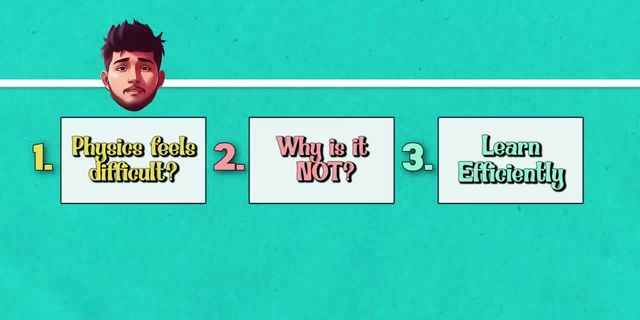 So first things first. in the next 7 minutes we'll discuss why everyone feels physics is very difficult, why is it not, and how you can become a pro at it. What is the exact step-by-step method to learn any physics chapter more efficiently? 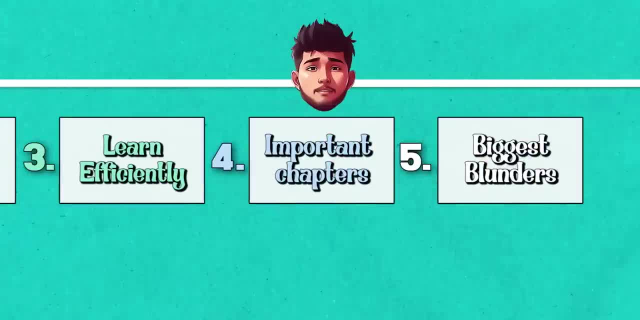 And then, if you're a JE aspirant, what are the most important chapters that you should solve first in order to score your best in JE mains and in JE advanced. And finally, we'll end this video with one of the biggest blunders that most of the JE aspirants commit. 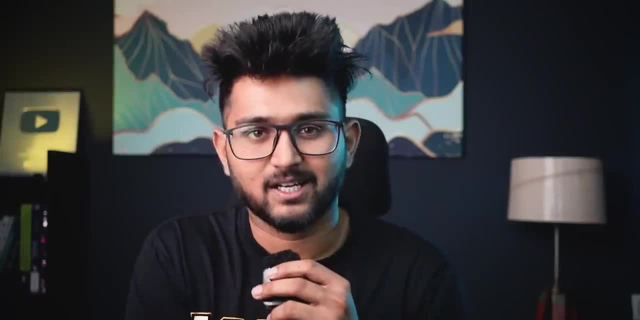 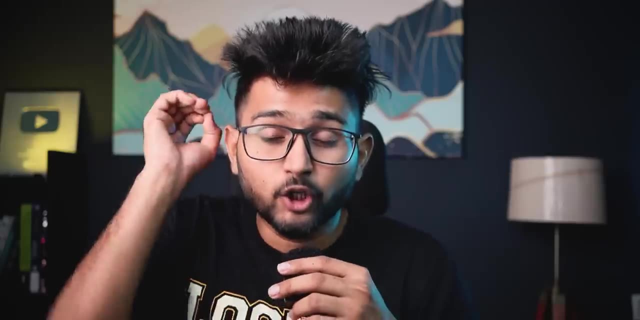 which you should definitely avoid. This video is going to be epic. Let's start First. why does everyone feel physics difficult? Simple, because it's being taught in the wrong And it's being learned in the wrong way. Most people just say: this is the axiom, this is the theorem, this is the derivation. 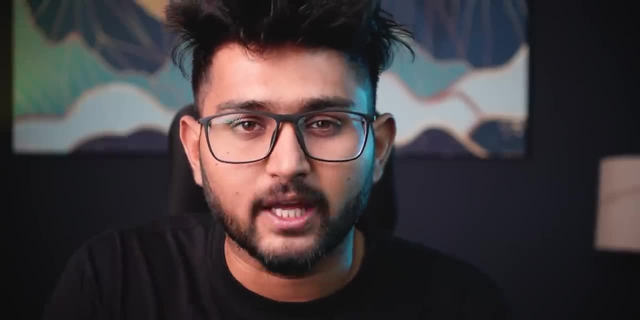 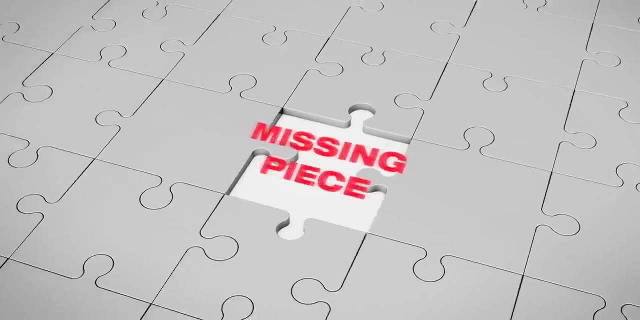 this is the formula that you should remember for the exam, But when a student actually goes to the exam, you didn't know what formula to use And, most importantly, you wouldn't understand why that exact formula is being used over there. It's like people just forget the missing piece which makes a physical chemistry question. 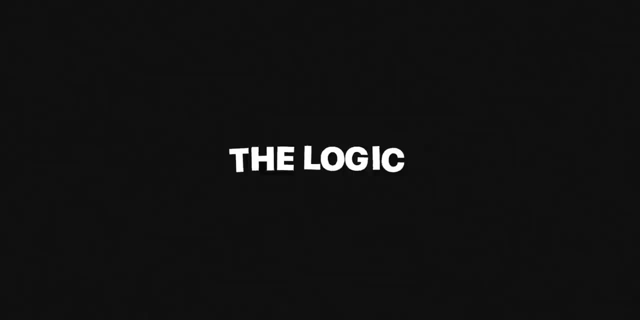 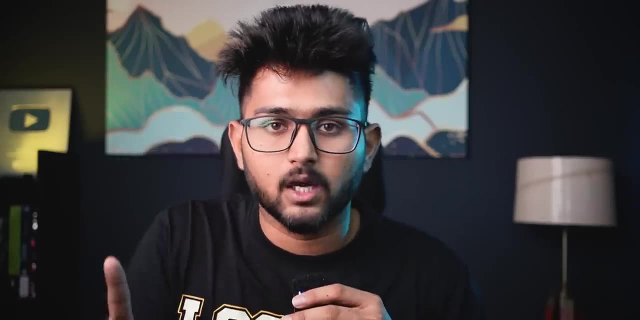 different from a physics question in JE advanced the logic. So, moving to the next point, how can you become a pro at it? I'll prove this point with an example in the next one minute, But first the method is simple. 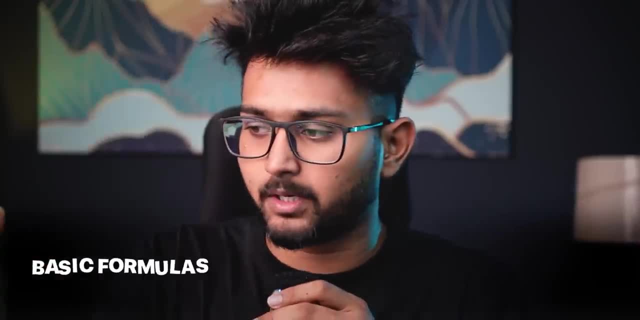 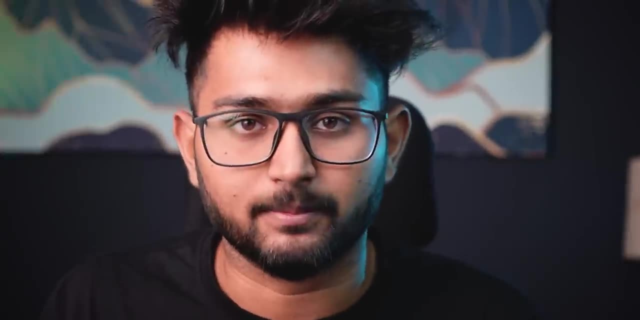 Instead of learning and mugging up all the formulas in a chapter, just learn the basic formulas, the basic theorems and the basic derivations in any chapter, Because these are the most important things while learning any concept. Now, the next skill that you should develop before solving any question in physics: 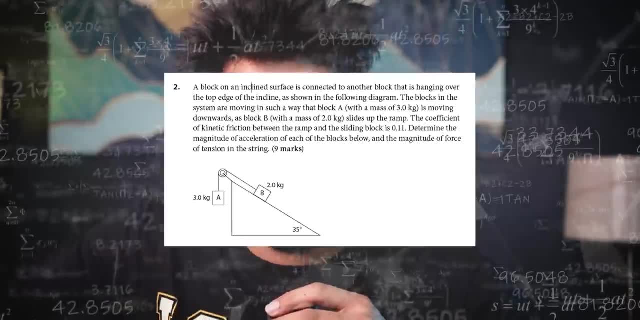 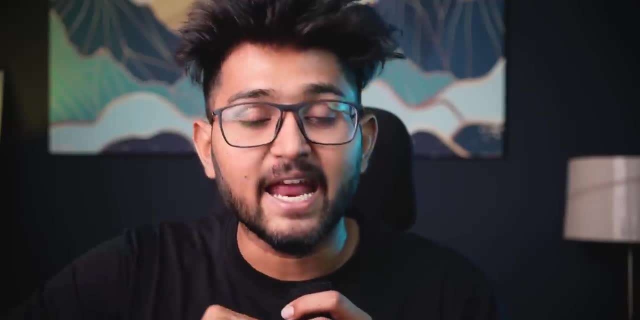 is to read and understand the question well. If you can break down the entire question into parts and apply some basic concepts between them, you're more than halfway done with solving the question. Now the last step to be able to solve any question in physics is to become a pro at mathematics. 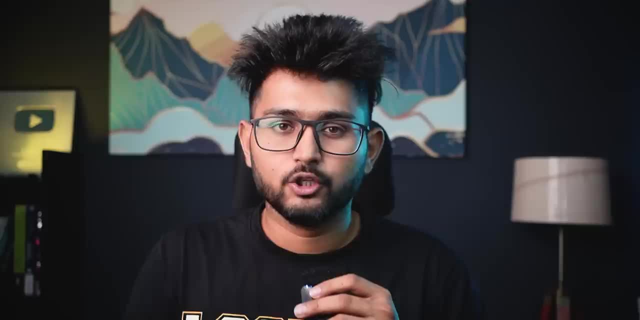 Because at a high level, every physics problem tends to become a maths problem. So you'll need to become good at maths in order to be a pro at physics. That said, if you can get these three basic things right, you're all sorted. 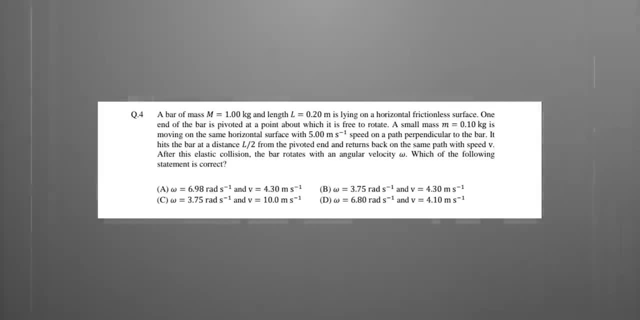 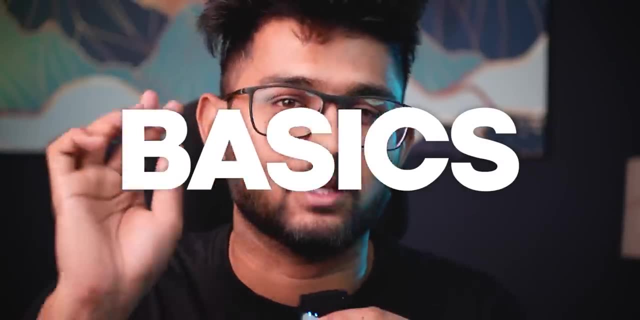 And to prove this point, let's take a small example question. This was the question which was being asked in JE advanced 2023.. And let me actually show you how easy it is. All we'll use is some basics and some logic. 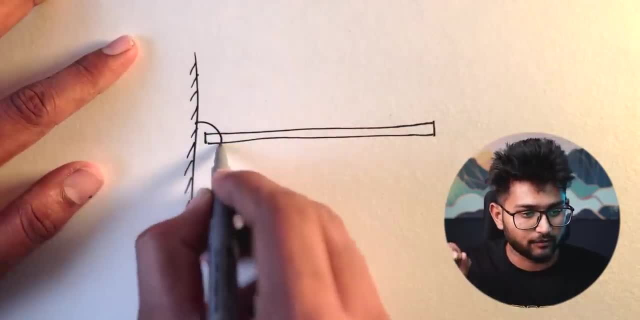 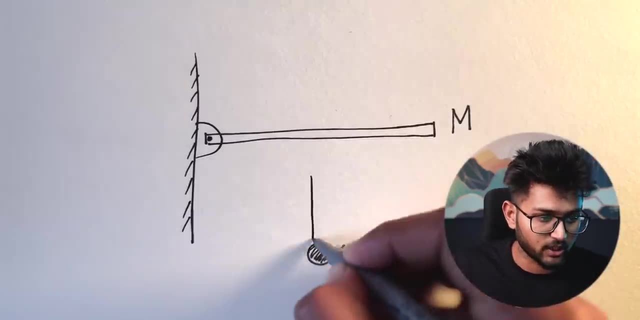 So here's the question. A bar of mass m and length l is lying on a horizontal, frictionless surface. One end of the bar is pivoted at a point about which it is free to rotate. A small mass m is moving on the same horizontal surface with a velocity v-naught on the path perpendicular to the bar. 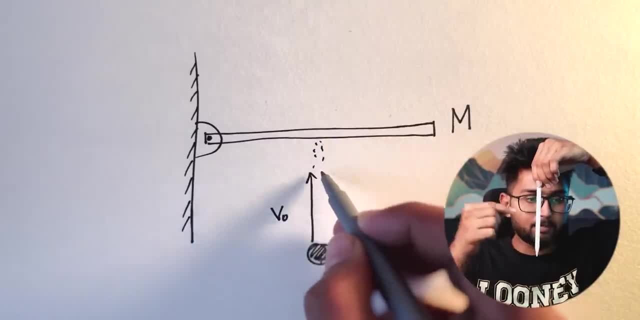 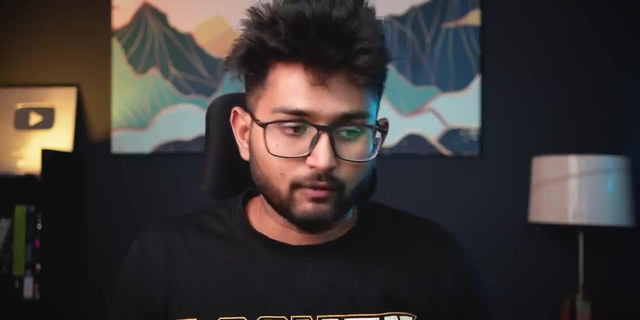 It hits the bar at a distance of l by 2 from the pivoted end and returns back on the same path with the speed v. After this elastic collision, the bar rotates with the angular velocity omega. which of the following is correct? So here we basically need to find the final velocity of the ball and the angular velocity of the rod. 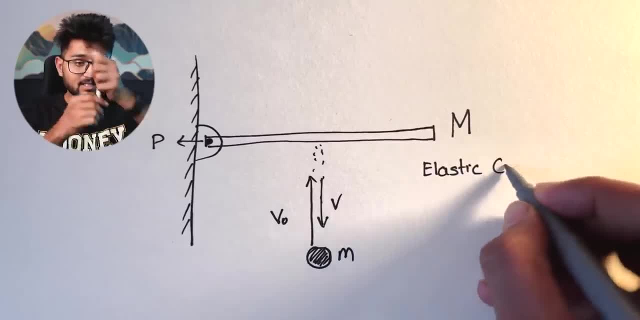 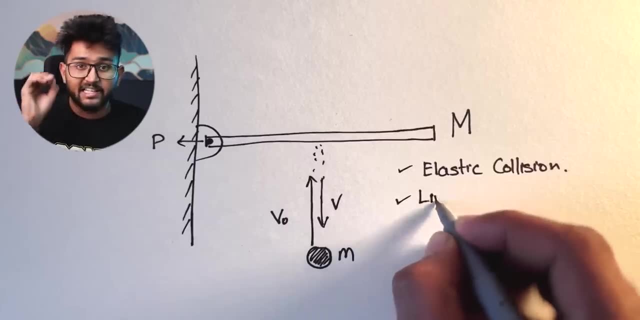 Right? So let's just go by the basics. So they gave that this is an elastic collision, which means energy is not lost, Right Right? So energy is conserved over here, And then we have the next thing, which is linear momentum. 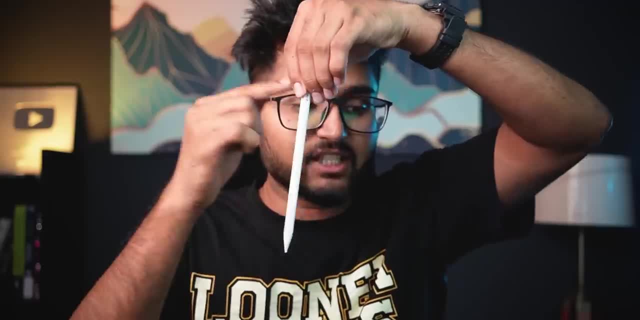 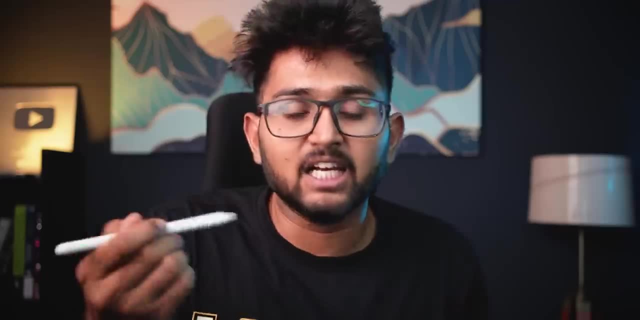 Is it conserved? No, it's not, Because there's a reaction force right When you're hitting this. there's a reaction force over here, which means there's an external force onto the system. And what about angular momentum? with respect to the point P: 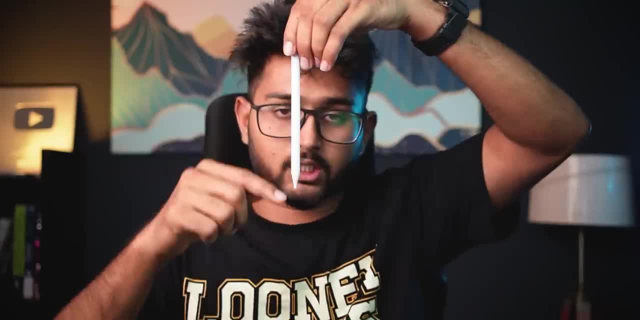 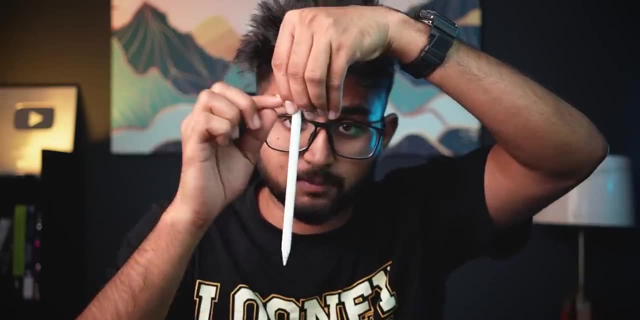 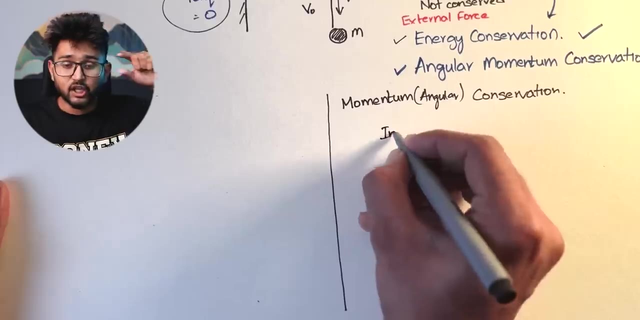 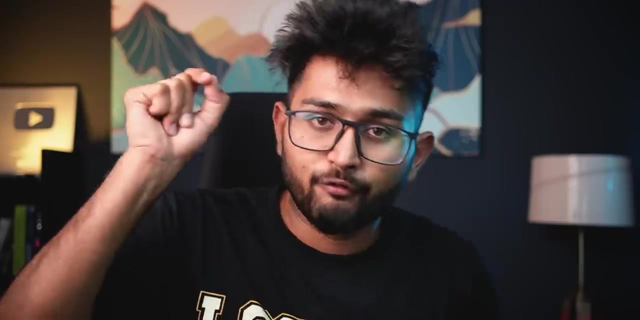 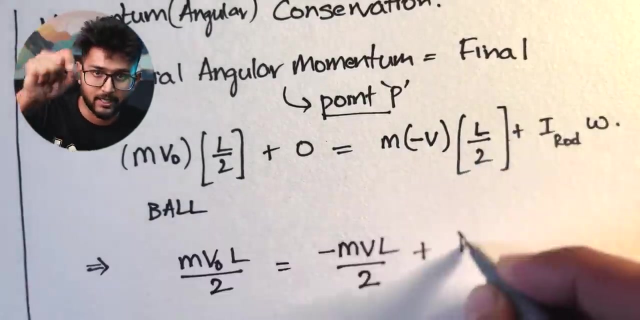 Is it conserved? Yes, it is Why? Because the torque across the point P is zero. So if the torque is zero, it means the angular momentum with respect to this point is conserved. So that's it done. First, we'll conserve the angular momentum with respect to the point P, which means initial angular momentum of the ball with respect to point P plus initial angular momentum of the rod, which is zero, is equals to final angular momentum of the ball plus final angular momentum of the rod with respect to point P. 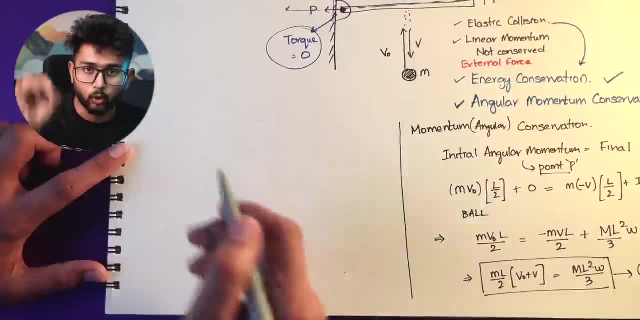 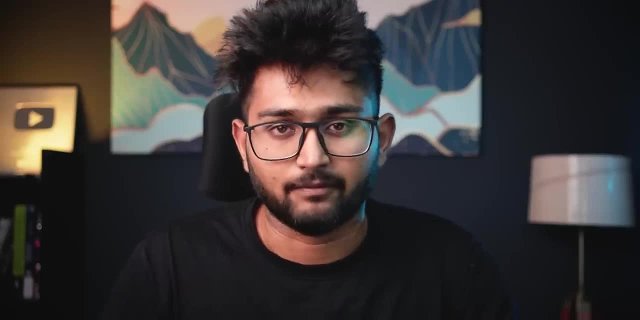 From there we'll get the equation number one and then we'll conserve the total energy of the system And from there we'll get the equation number two. So once we got these two equations, it's just mathematics after that. It's a very simple question. 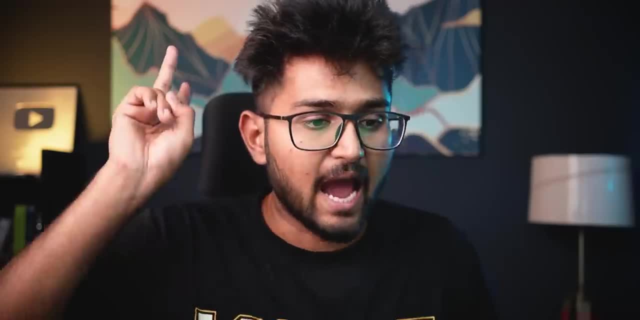 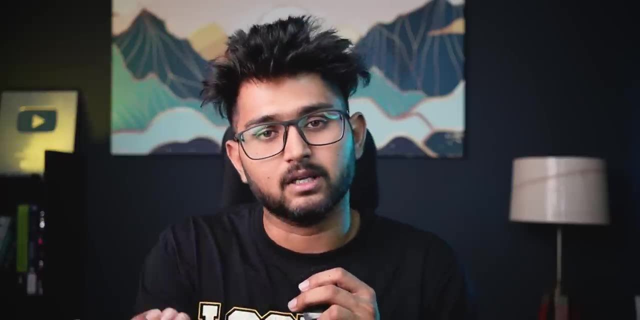 If you know the basic definitions of momentum, force, angular momentum and torque. And this is the question asked in JE Advanced 2023.. So that is it. It's simple: Basic concepts and formulas plus some basic logic, plus mathematics is the way to succeed in physics. 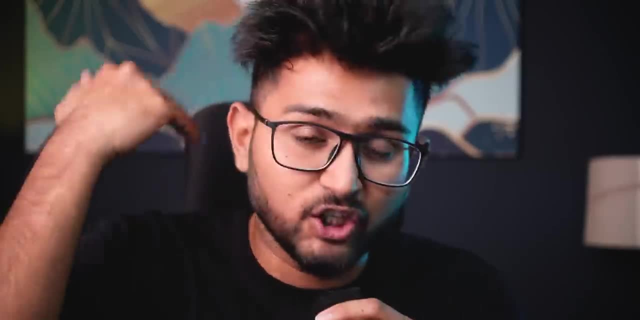 And now, as you got a proper clarity about why people find physics difficult and how can you become a pro at it, now let's discuss the step-by-step method in order to become a pro at any chapter in physics in the next one minute. 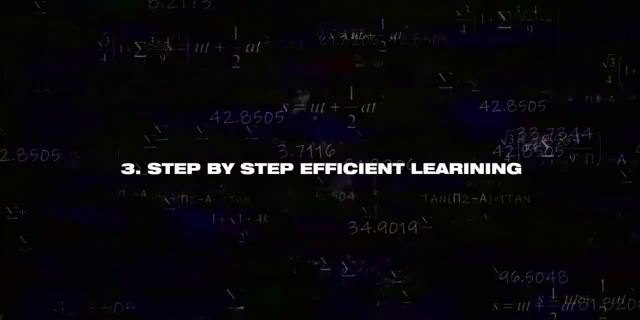 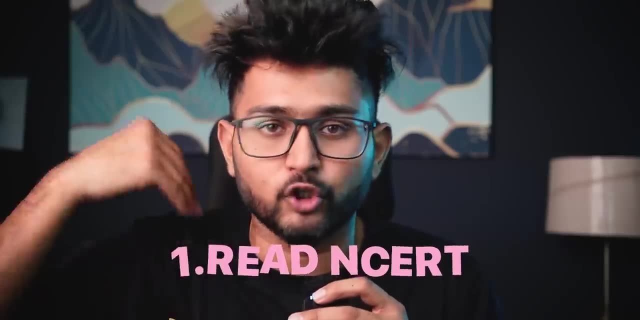 And then we'll talk about the most important chapters for JE Mainz. So let's get into it. So let's start. This is the exact step-by-step blueprint of it. The first step is to start reading and see it, even before you listen to the class. 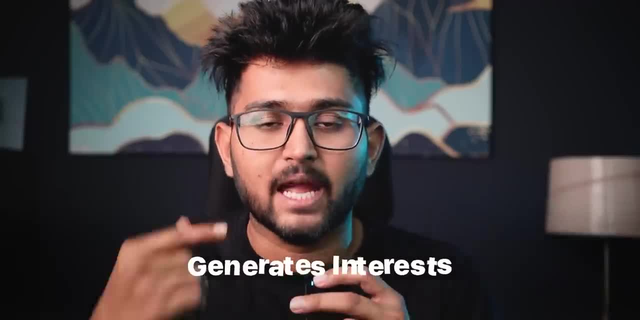 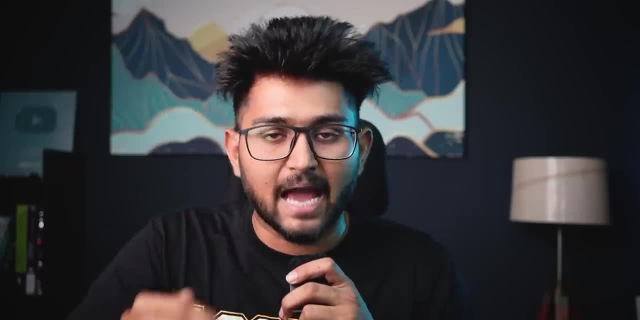 They set up the basic understanding of the concepts, generates interest and also raises some preliminary questions in your mind. The second step is to listen to your classes, and all the questions which are being raised in the first step will be answered if you listen to your class as well. 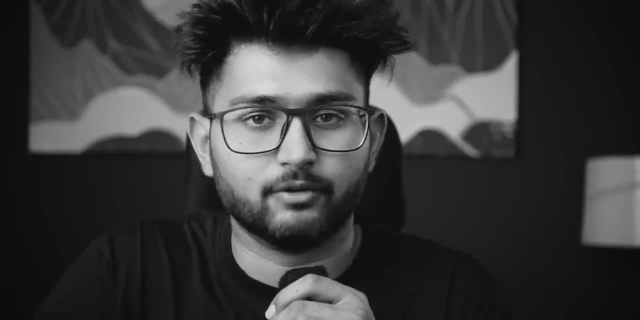 See now, if you just have three to four months left, I'm so sorry, but you won't be able to finish the first two steps. So instead of that, skip both of them and just watch one shot. Let's go. 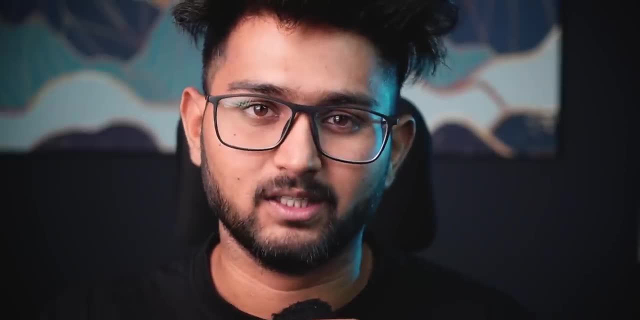 So what you're learning in this step is that you need to do one or two lectures on YouTube for every chapter. That's the only thing that you can do properly. So once you're done with the step one and step two, the next step is to solve some example questions from either HC. 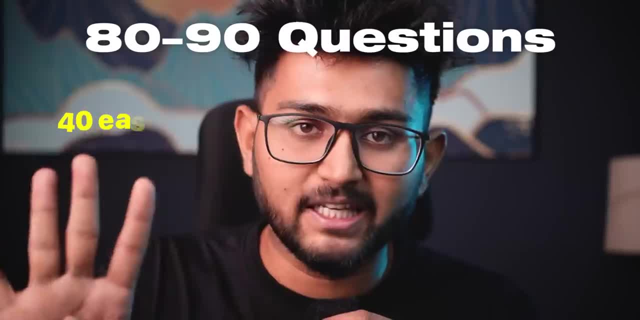 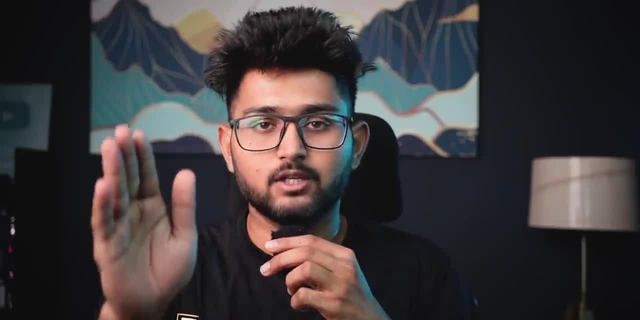 Verma, Cengage or Physics Galaxy, and then solve 80 to 90 questions from each chapter- 40 easy, 30 medium and 15 difficult- either from your study material or from any of the standard book, And finally, solve some previous year questions and you'll be good to go. If you do all these things right, you'd be able to finish your JE Mainz preparation in something around three to three and a half months, plus marks in physics, and you'll take something around six to seven months for your JEE advanced. 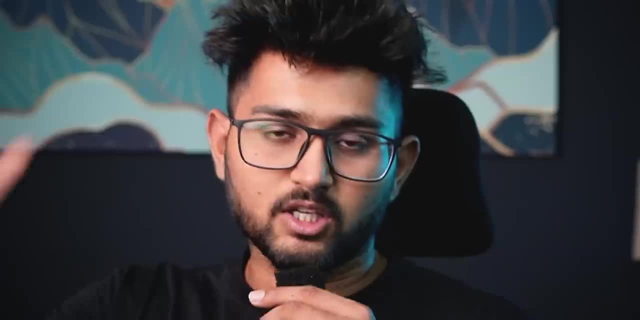 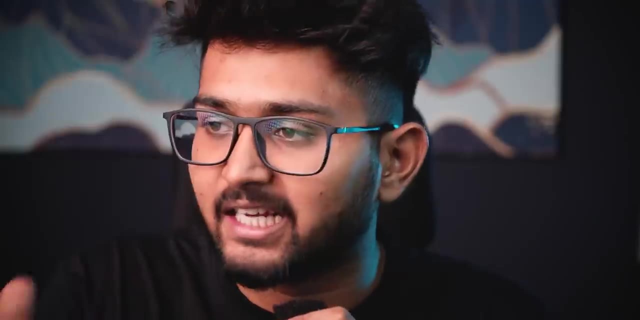 preparation and end up scoring something around 60% to 70%. This is my guarantee. So now, before we end this video, let's look at some of the most important chapters, both for JEE mains and JEE advanced, so that you can start your preparation in the right direction. set your priorities in the 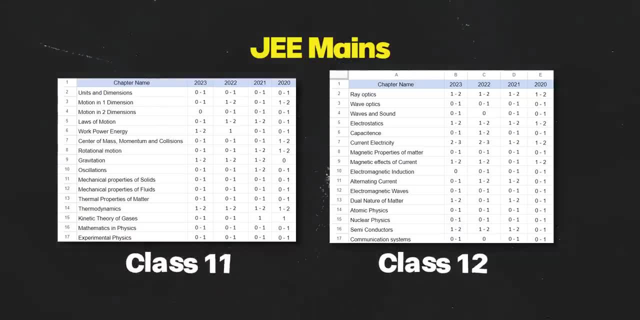 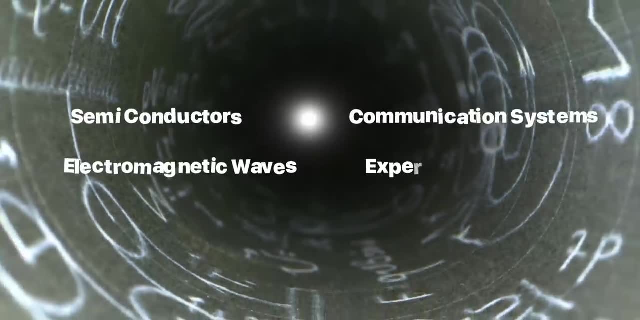 right direction. This slide that you see on the screen right now is for JEE mains. take a screenshot of this right now, because it is going to be very useful going forward. and for JEE mains I'd say: semiconductors, communication systems, EM waves and experimental physics are some of the easiest. 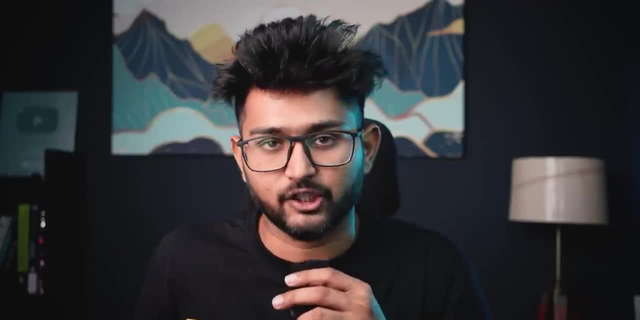 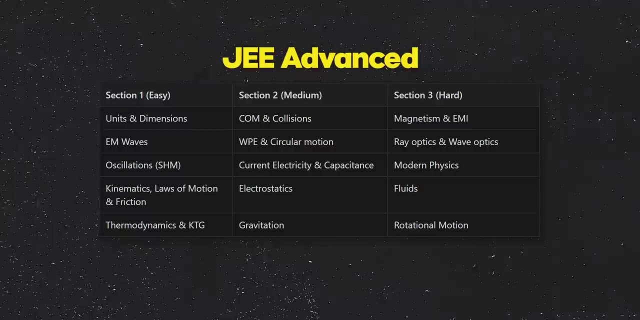 and most important chapters that you should definitely finish. You can easily answer four to six questions if you know these concepts well through NCRT, and this slide that you see on the screen right now is for JEE advanced. take a screenshot of this. this has the easy medium and 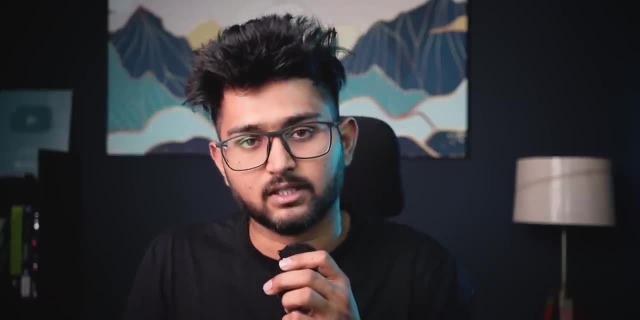 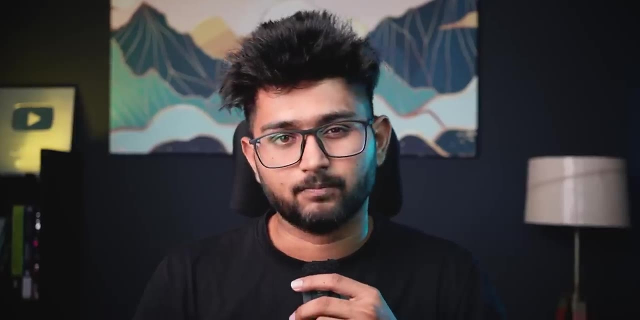 most difficult chapters, which also have heavy weightage in JEE advanced. Start from the easy chapters, because that will give you the initial momentum and will also help you build confidence in you Got it. Physics is easy. all you need to do is to get the basics right and apply some logic. 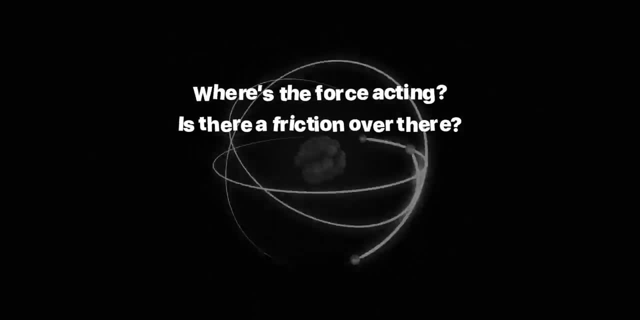